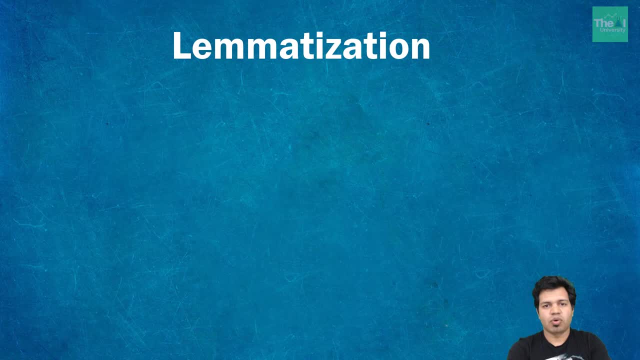 lemmas or lemmatah is the canonical form, citation form or dictionary form of a set of words. In order for a lemmatization to resolve a word, it is important to have a set of words which are the basic الم and its lemma as a whole. it is also important to know the part of the lemma. 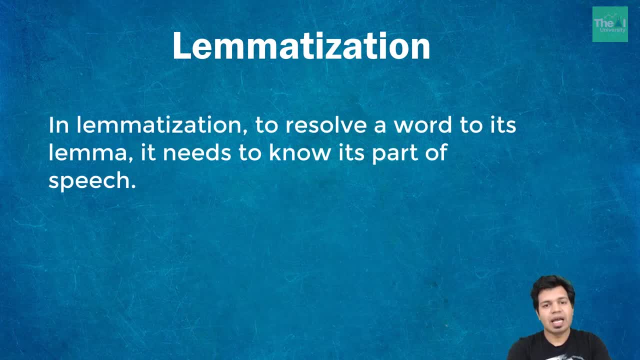 In lemmatization, a word needs to know the part of the speech which actually requires extra computational linguistic power, such as a part of speech tagger, and that's the whole reason. lemmatization resolves a word to its lemma in a better way, For example, resolving: 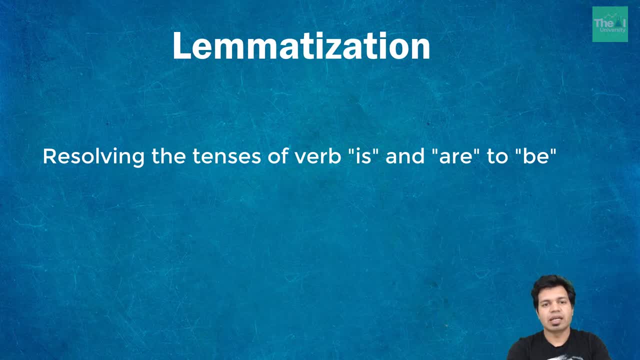 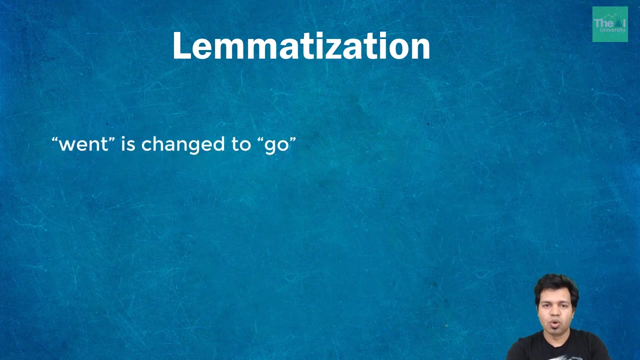 is the word is and are is to the word be, are to the form be or to the form be and are be. okay, for in simple words i can say that verb verbs in past, past tense are changed into present. okay. example went is changed to go and synonyms are unified. example best is changed to good. 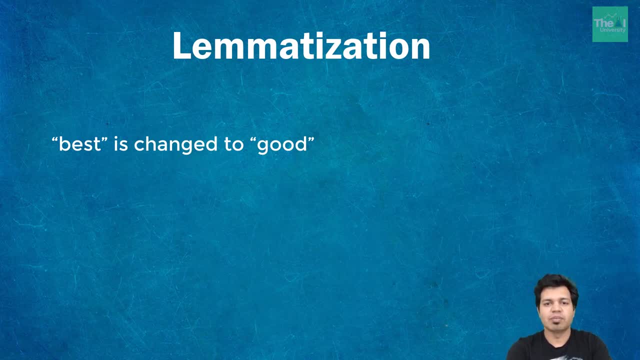 hence standardizing words with similar meaning to their root. so the important thing is that lemmatization requires a part of speech tagger. okay, although it seems closely related to the stemming process, lemmatization uses a different approach to reach the root forms of words. let me take one more example here: the words caring and cares. 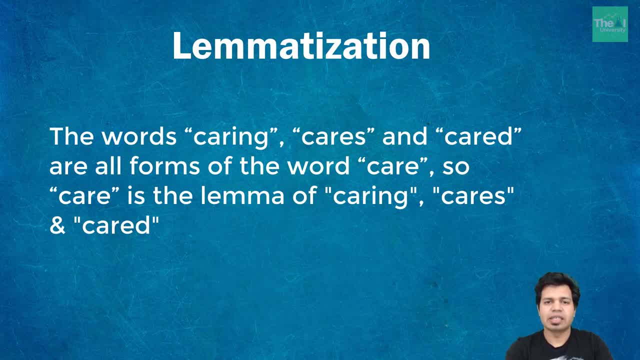 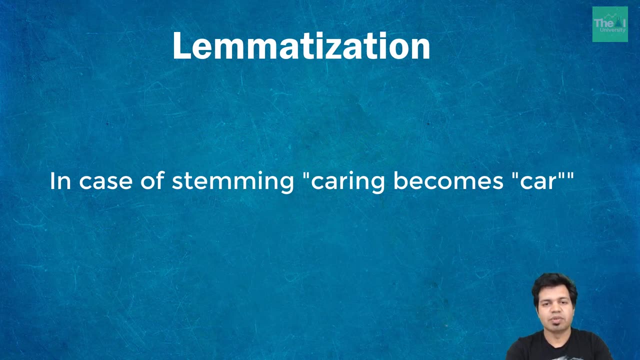 in fact, caring, cares and cared are all forms of word care. so care is the lemma of all the previous words, whereas in case of stemming, caring becomes car. okay, so that's the difference between these two, because, uh, lemmatization is using part of speech, tagging here. that's why it is giving you a right form. 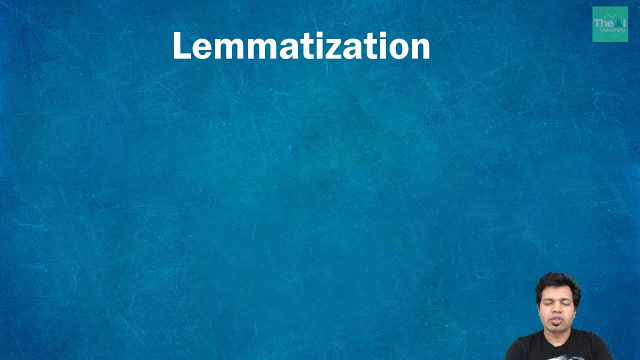 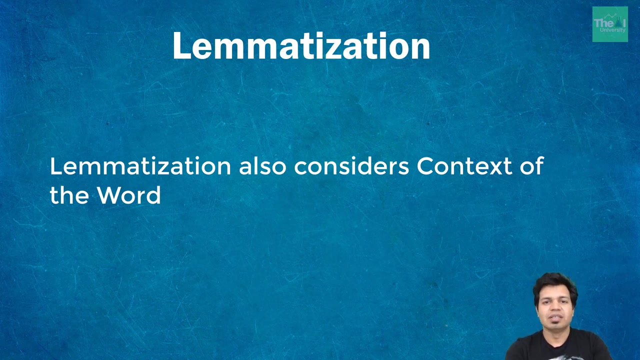 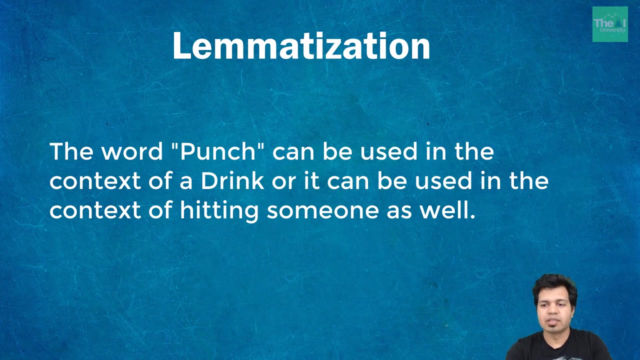 or right lemma. lemmatization also takes into account consideration: uh, the the context of the word, which means it can discriminate between identical words that have different meanings depending upon the specific context. so think about words like punch, which can correspond to drink as well as to hitting someone. okay, then we have another word: uh. 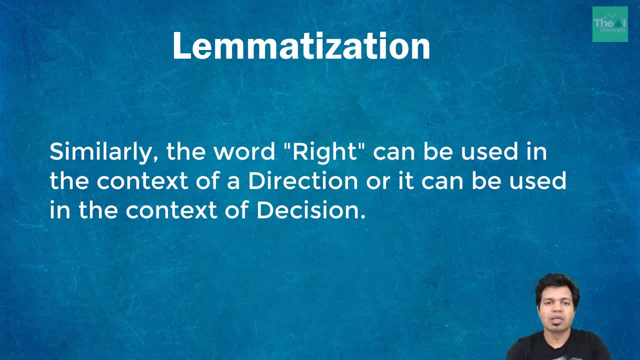 like right, which can be used for direction like right or left, as well as for decisions like right and wrong. so, in a nutshell, lemmatization is much more resource intensive task than performing a stemming process. also, it requires more knowledge about the language structure than a stemming approach. 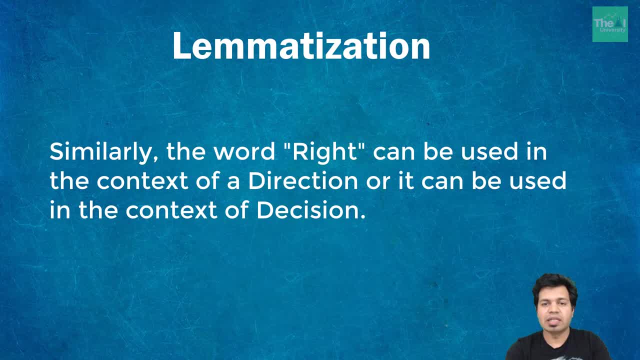 it demands more computational power as well than setting up or adapting a stemming algorithm. so let's move on to the python code for lemmatization. please note that python nltk provides word net lemmatizer that uses the word net database to look up lemmas of the words. so let me open. 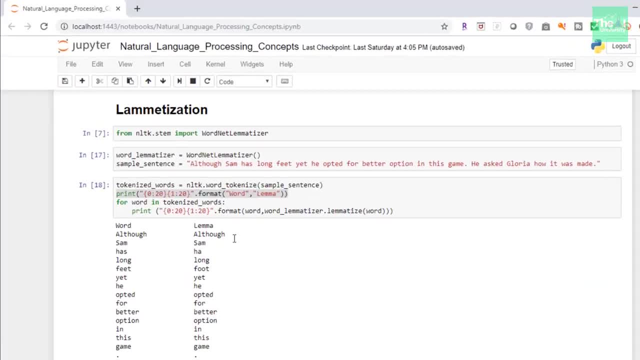 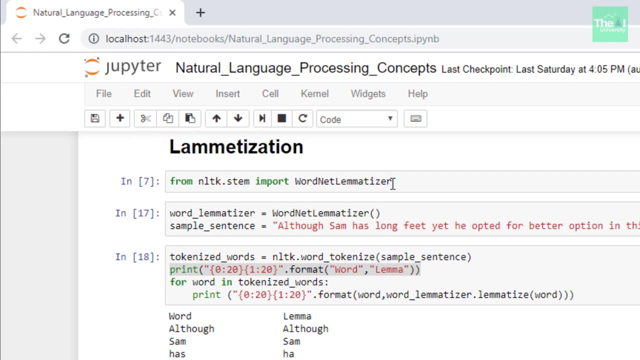 my jupyter notebook real quick here. okay, so in the first cell i'm importing word net lemmatizer which can, which you can see here, and this is a class from nltk dot stem package. and, uh, in the next line i'm creating an object of word net lemmatizer here. okay, so this line, in this line, i'm just creating an. 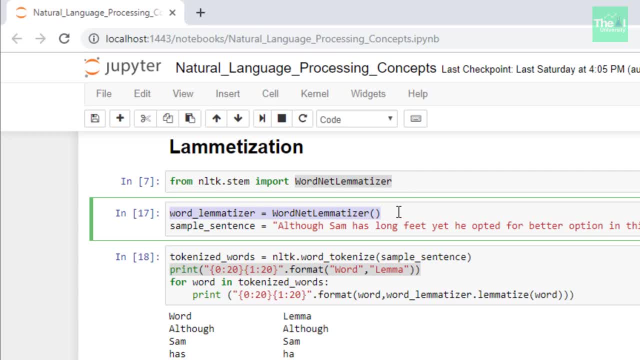 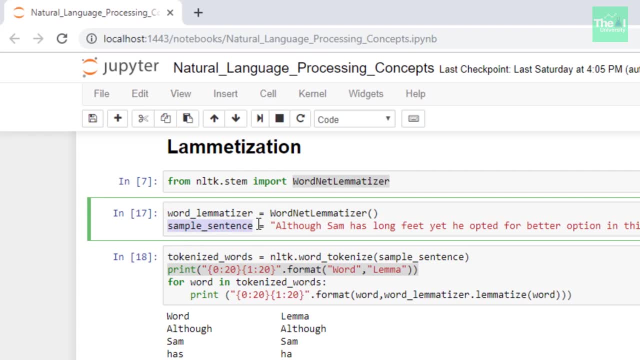 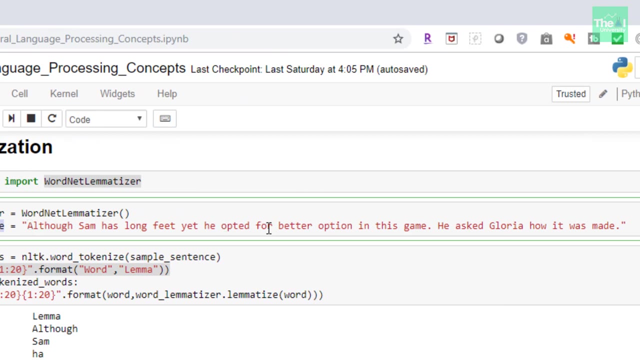 object of word net lemmatizer. okay, and i just stored it into this variable word lemmatizer. after then, i created a simple sentence: uh, in order to play around uh. and the sentence is: although sam has long feet yet, he opted for the better option in his game in this. 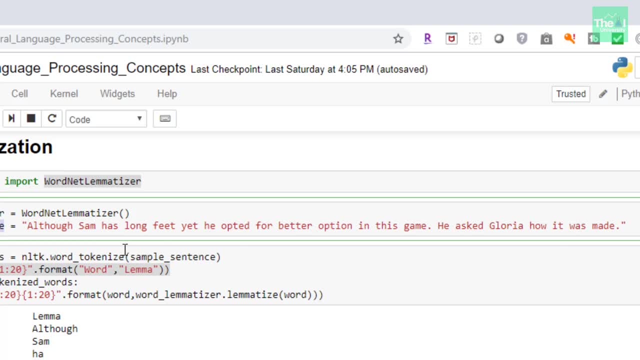 game. he asked gloria how it was possible to get a bad location on his turf and in fact he asked sam. he means to create three different trees with short axis. so in order to do this was made okay, so in the next cell, I first tokenized the sentence into words. 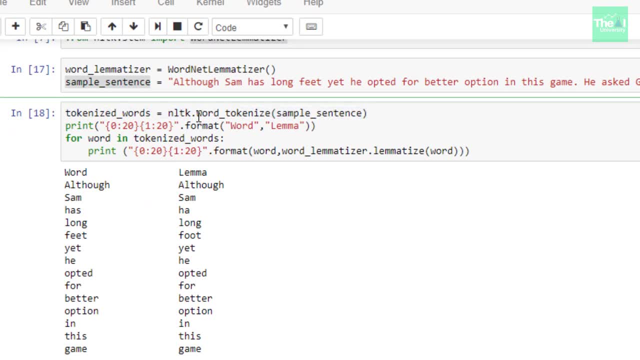 using this sentence so you can see the word tokenize I'm using here and passing this sample sentence as an argument. okay, and then I used a for loop. okay, for basically to go over each of the word in the tokenized word list. so this is the word list, tokenized word list, and I wanted to go over each and every word. 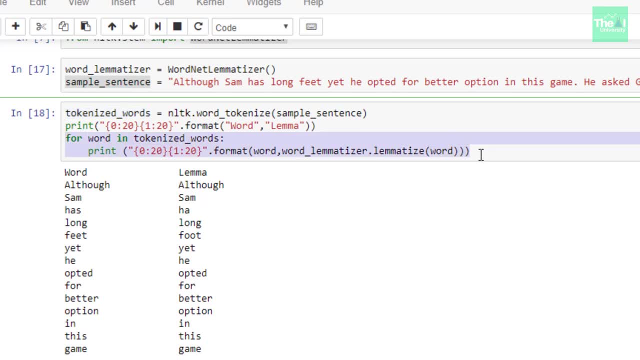 okay, so that's why I used a for loop here. okay, this sentence is nothing, but I'm just creating some headings here. so first heading is actual word- actual word. so first this represent the actual word and the second column represents the lemma associated with this word or the lemma form of the actual word. 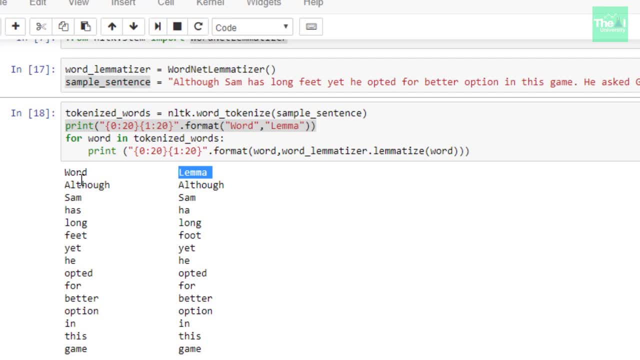 okay, all right. so if, in case, you don't know the usage of this dot format, let me tell you about the same. dot format is one of the string formatting methods in Python 3 which allows multiple substitutions- okay, and value formatting. so, multiple substitutions and value formatting. this method lets us concatenate, basically, the 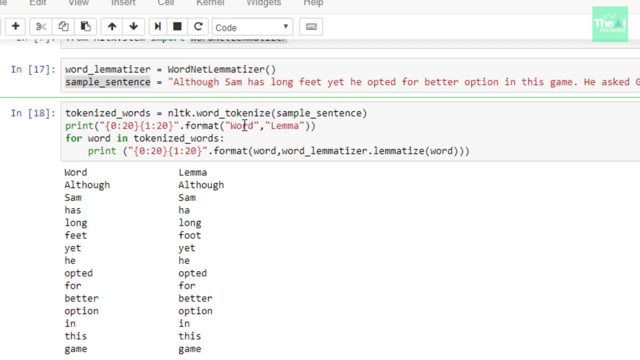 elements within a string through positional formatting. so here in numbers, these numbers within the braces it depicts alignment codes. ok, so that's what I'm doing here. I'm just fingering over each and every word in this tokenized word list and then I'm creating the world. lemmat Soups here. so this column is a word. lemma tizer, the. 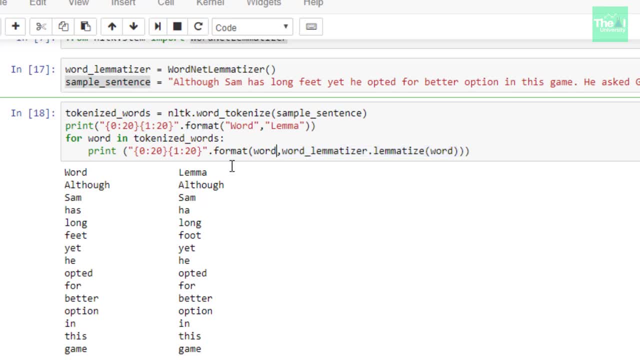 lemma tized world of actual world and this column is actual world. so now I'm going to go through all these ideas. we're going to go through all these ideas, we're so. this is the actual word which is represented by this and this is the. this lemma column is the. 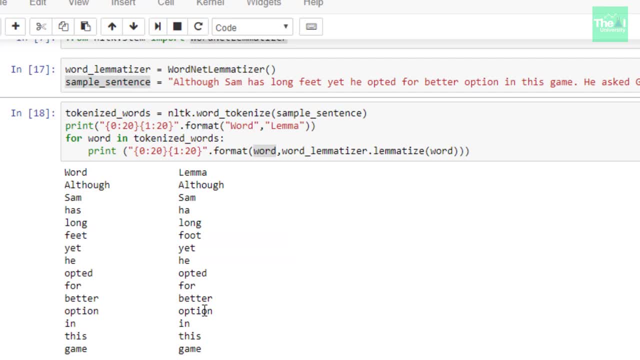 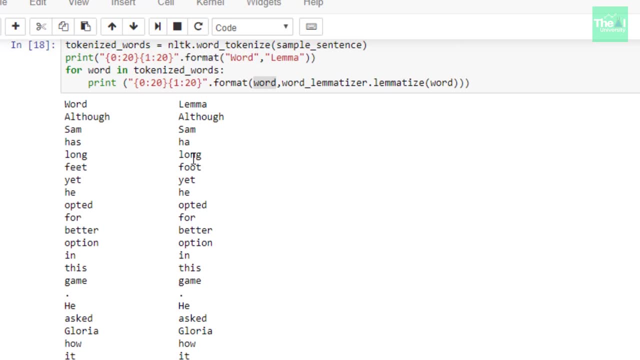 lemmatized word, okay. so when i ran the cell, let me see what is the output here. you can already see the output here. okay, so you can see the output here now. you might be wondering why there is no actual root form given by any word. so although is, although here sam is sam, long is long, okay. 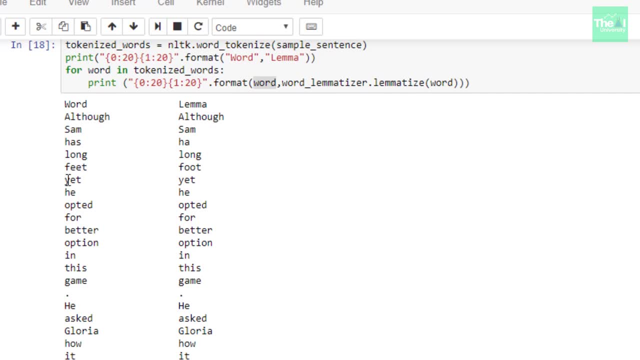 feet is changed into foot, yet is, yet he is, he opted, is opted. so majorly, most of the words are not changed at all. okay, and basically the words are not lemmatized to the actual root form. okay, and the reason for that is there, because we have mentioned, we haven't mentioned any part of speech tagging. 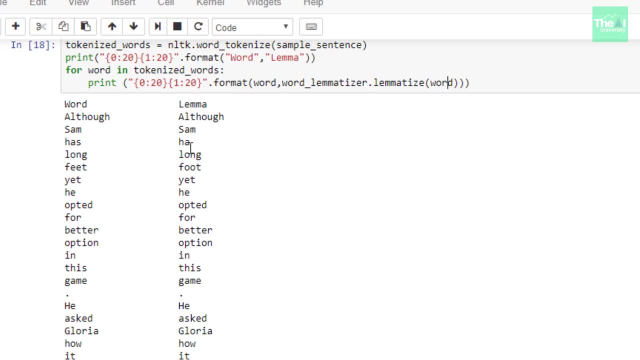 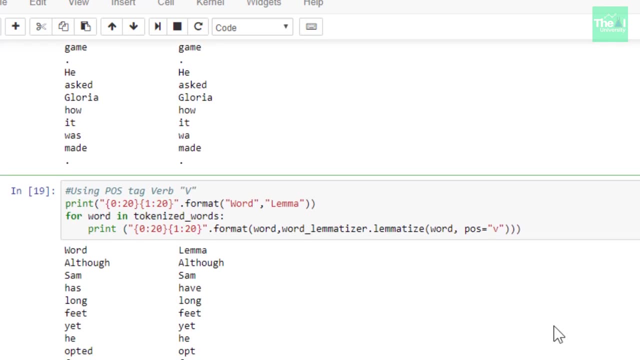 here. okay, that's why it came as just like that, just as it is only okay so if I make a tweak little bit in this. so I just passed another argument here which is part of a speech and here we represent verbs, okay, so when I ran this, 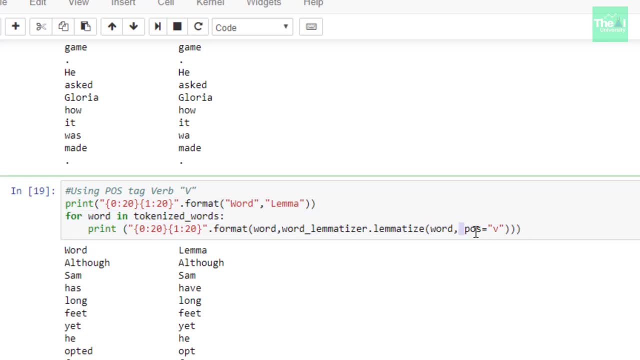 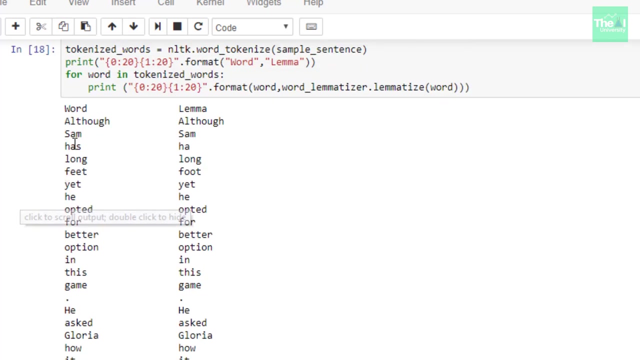 particular code, once again providing an additional argument which is part of speech. equals to V, V is. well, then you can see a variable changes with the verb, with the words which has some verb form. okay, so you can see has is changed as have, whereas earlier it was not changed. I think it was how right. 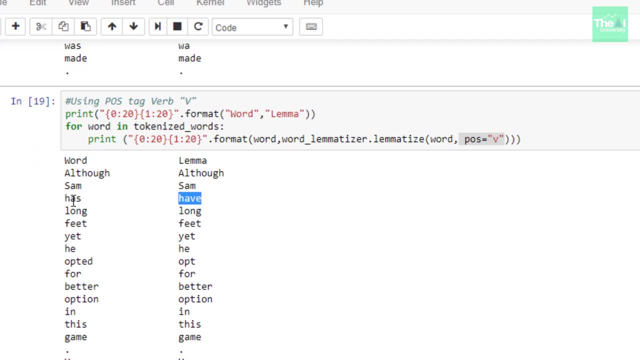 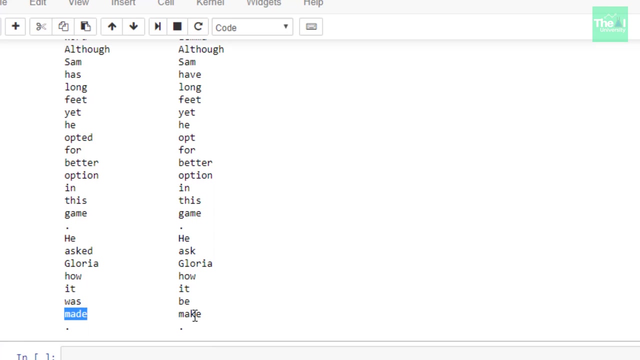 so so has has been changed. so has is a verb form of the word. so it has been changed to have okay and then opted is changed to opt. then what else you can see? made, the word made, which is a verb form, again is changed to make okay and was was. 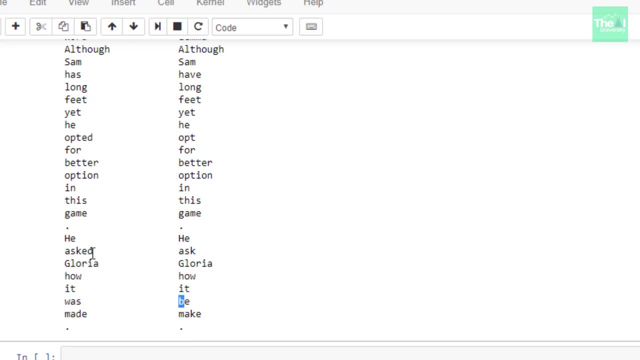 changed as be. you can see very well again. ask, just changes. ask, okay. so you can very well see that the word got lemmatized to his actual word. okay, keeping in mind the part of the speech as well. okay, now the million-dollar question comes. when do we use a stemming? 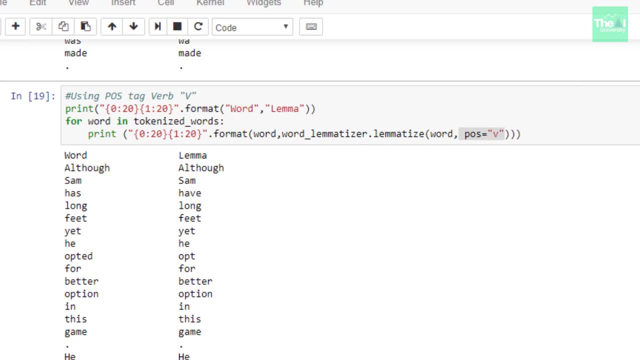 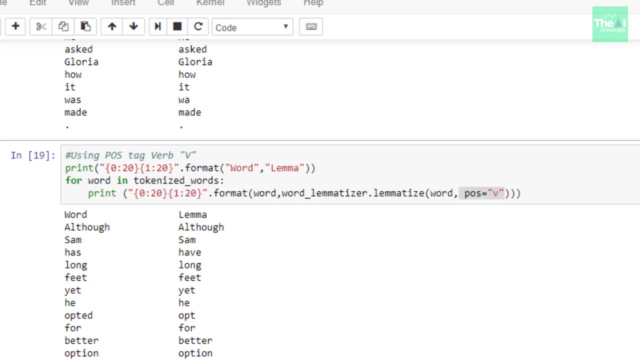 and when do we use lemmatization? okay, well, it actually depends upon the application you are building, which can govern whether stammer should be used or the lemmatizer should be used. if speed is of prime importance, then stemming should be used. otherwise, lemmatizer can be used in place of that, because 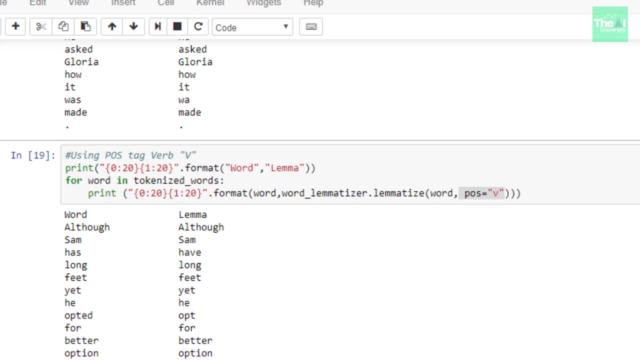 lemmatizers can scan a corpus, which consumes both time and processing. okay, so if you are building a languages application in which language is a language is important, then you should use lemmatization, as it uses a corpus to match root forms. okay, so, folks, this is it for this video.